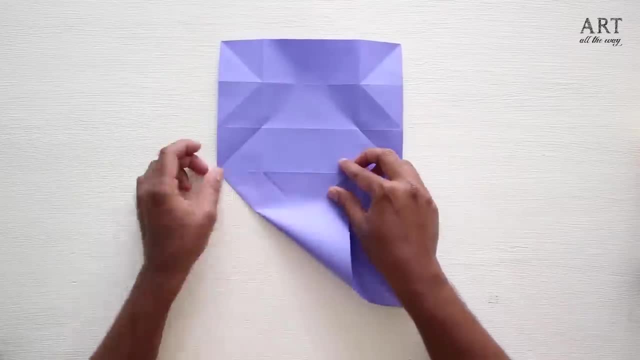 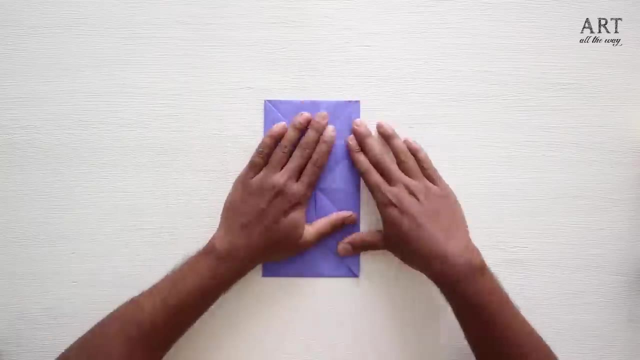 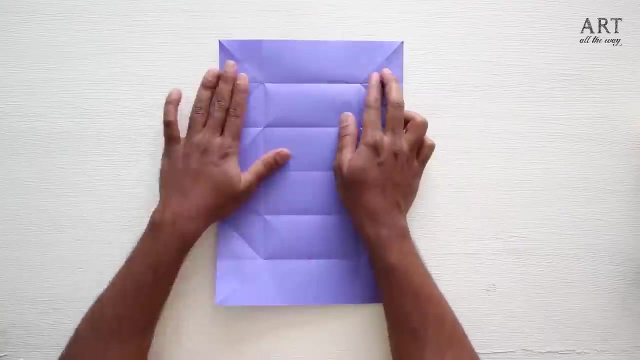 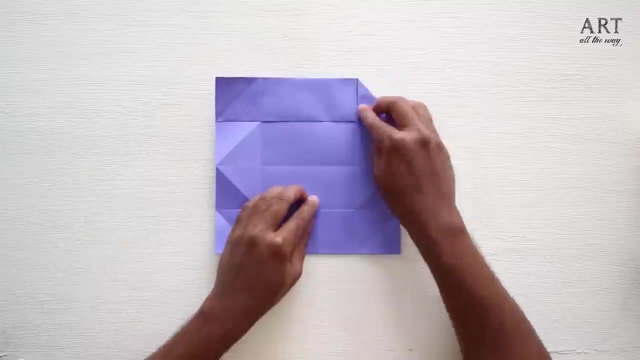 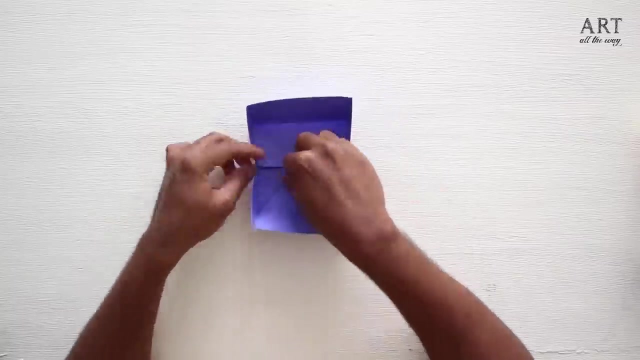 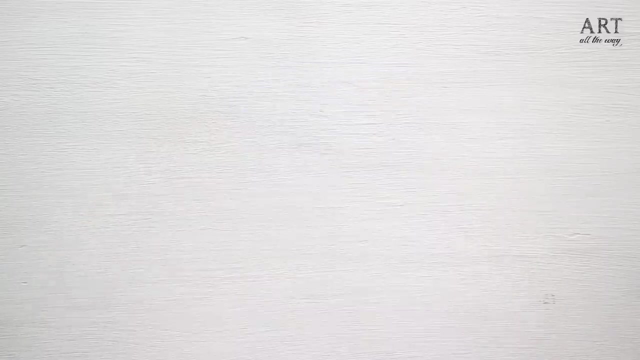 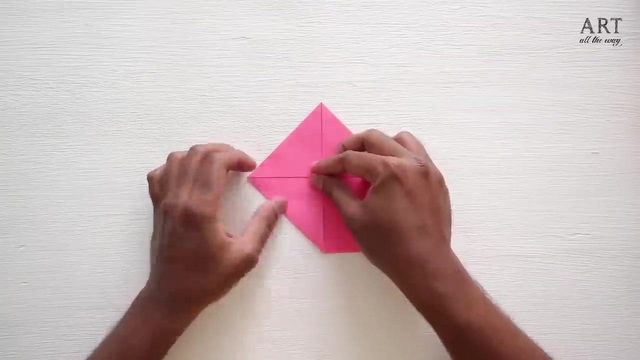 And then they took a rest or walked over and they fled. You wrote to me. you wrote to me: this is Annalie Cause she wanted me. this is Annalie Cause she wanted me. this is Annalie. She kept quiet. they kept beating her. 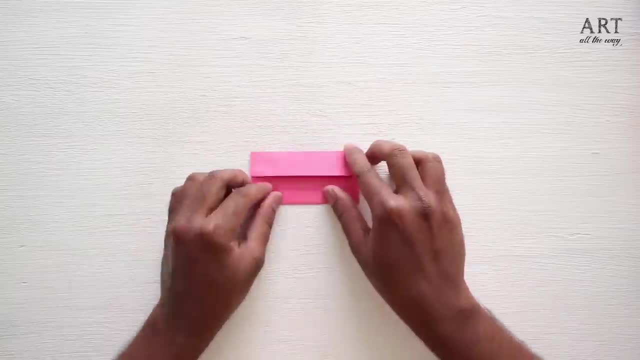 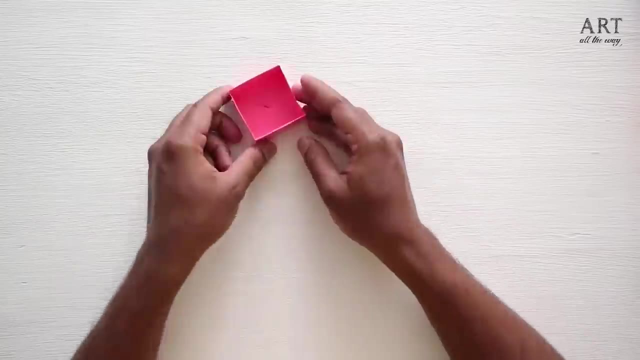 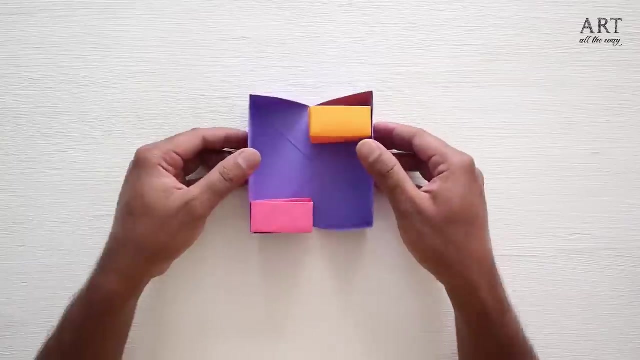 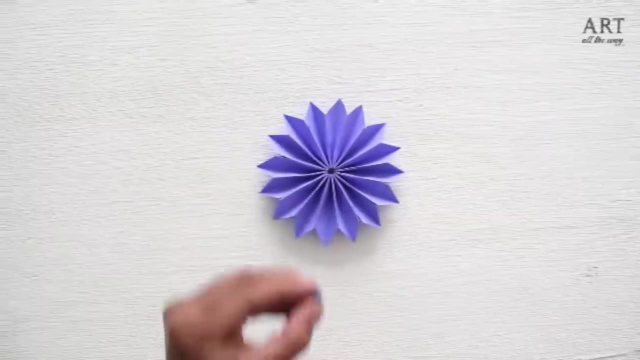 They felt sad for her. But an order is an order. She was a prisoner There in the dark. there in the dark, There in the light, She stood, But she knew they couldn't break her. And by the shore, the bombs were falling with the snow. You wrote to me. you wrote to me. this is Annalie. 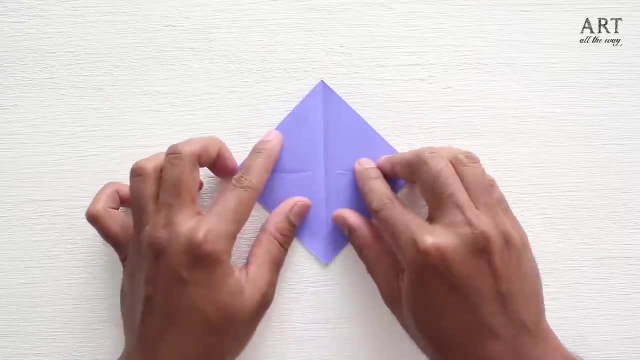 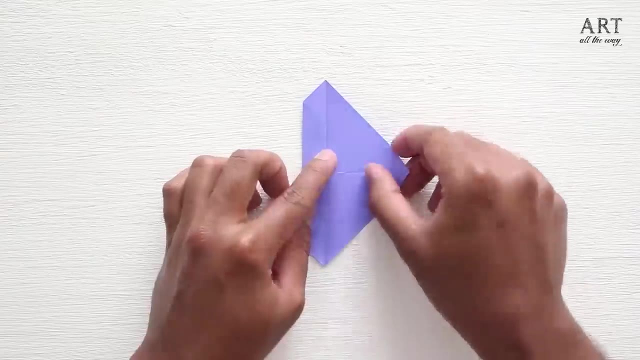 You wrote to me. you wrote to me: this is Annalie. You wrote to me. you wrote to me. this is Annalie. You wrote her a G Six And maybe it was just love, Maybe she don't care, Maybe she'm fine. She was a good nut. 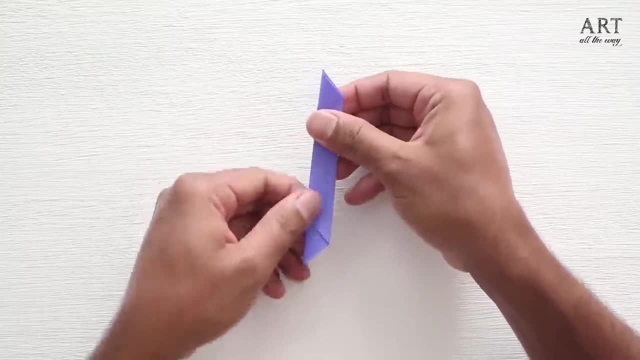 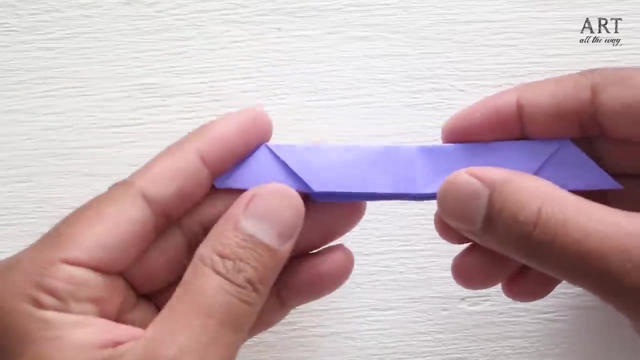 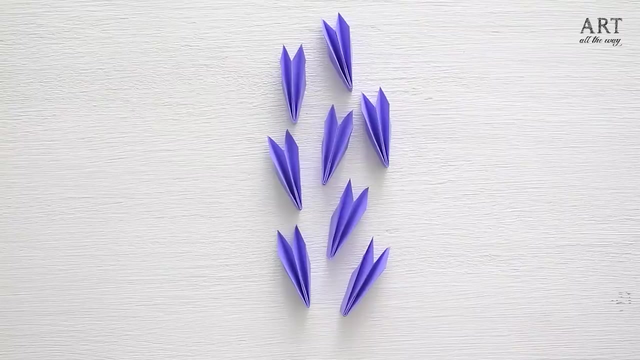 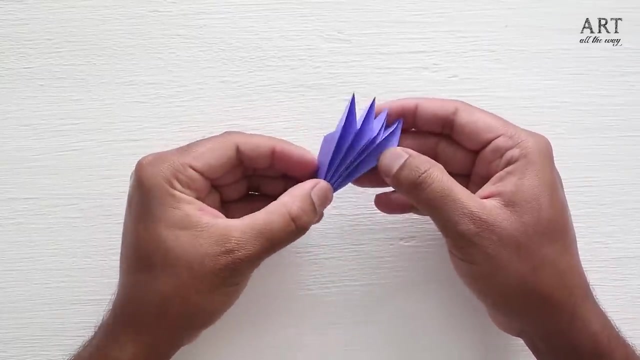 You told me always She doesn't get hurt The sweat on your cheek, Can a closer look? Cause she wanted me. This is Annalie. Cause she needed me. This is Annalie Cause she needed me. This is Annalie Cause she wanted me. this is Annalie. 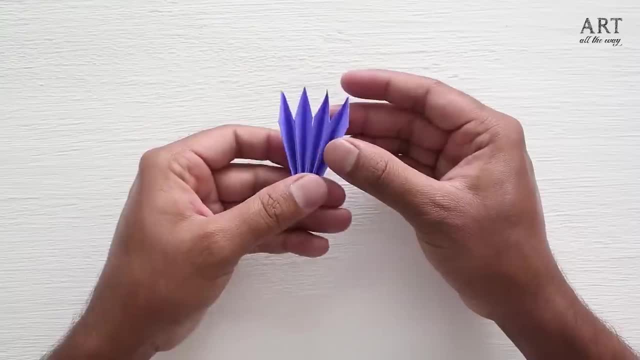 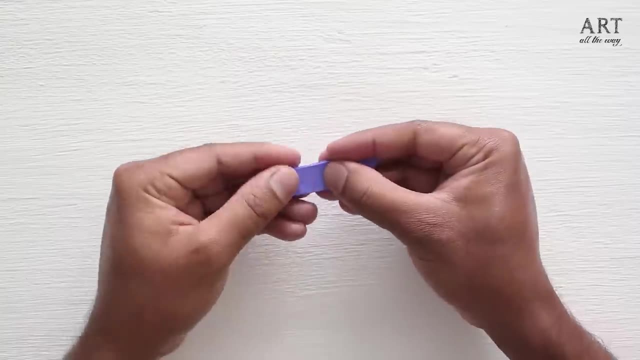 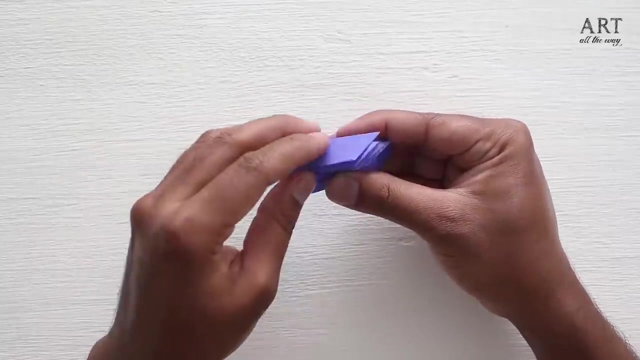 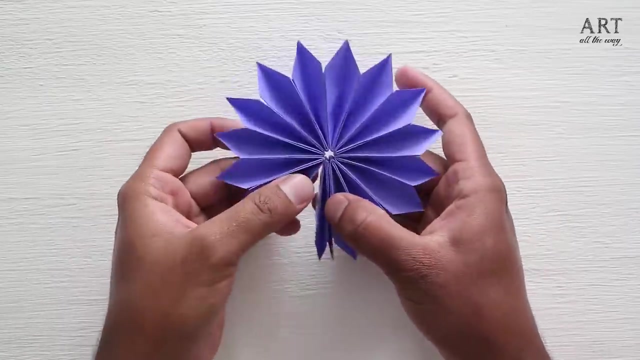 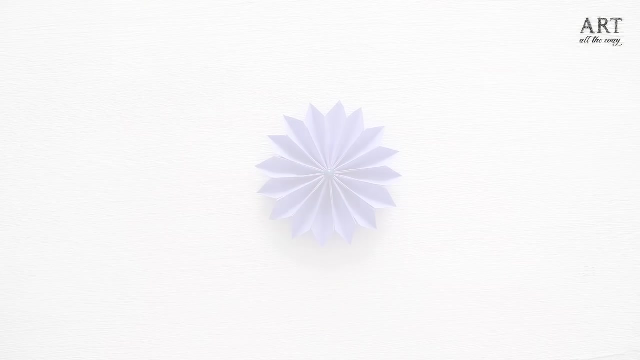 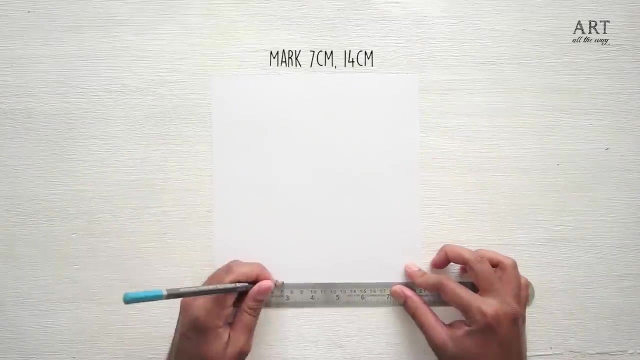 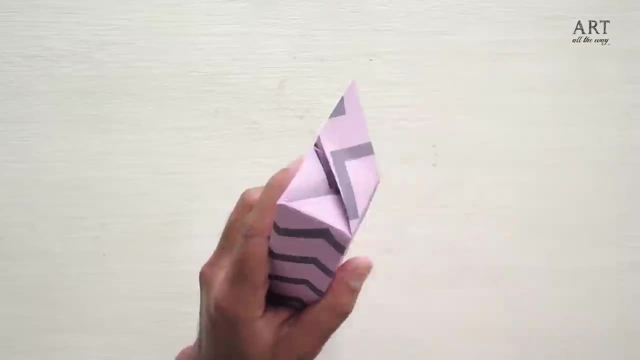 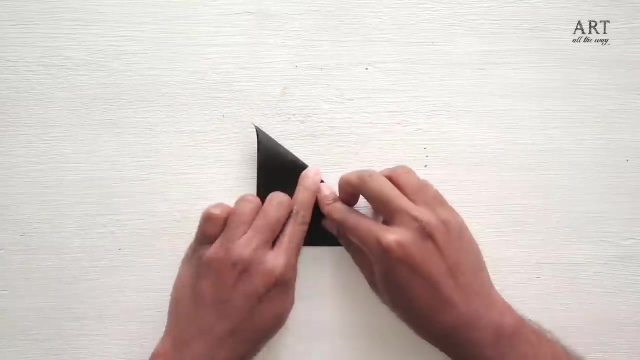 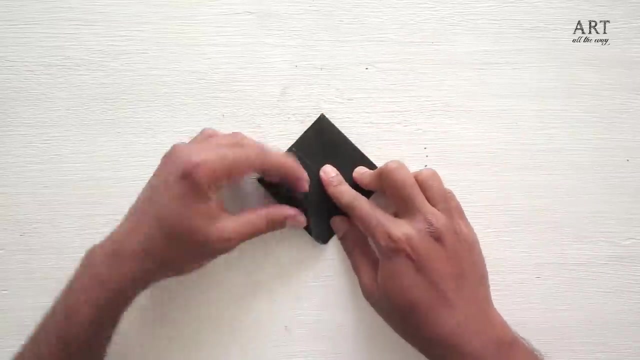 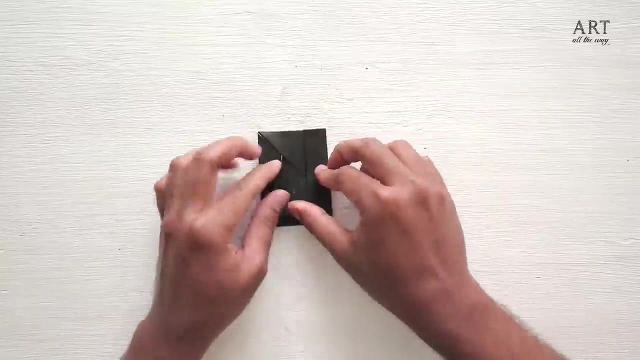 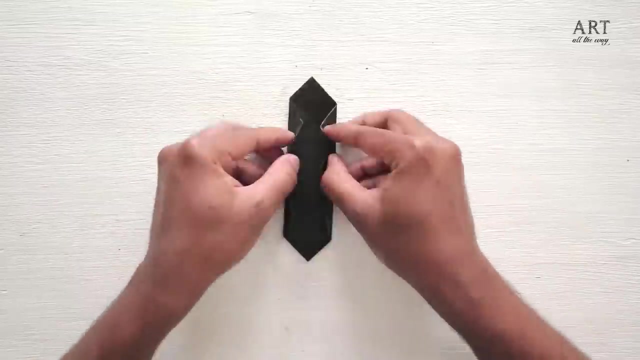 I was running from myself those days, Always breathless search for something safe. And then I smashed into that golden face For the first time. I don't run away. We danced together till we got it right. Ups and downs through many days And nights, But you appeared to be my guiding light. And at the same time I realized: Oh, baby, when you hold me, I rather lost my senses Than be lonely. Cause, baby, when you touch me, I feel holy. Oh, nothing in the world would, Oh, would, kill me As long as I got you. 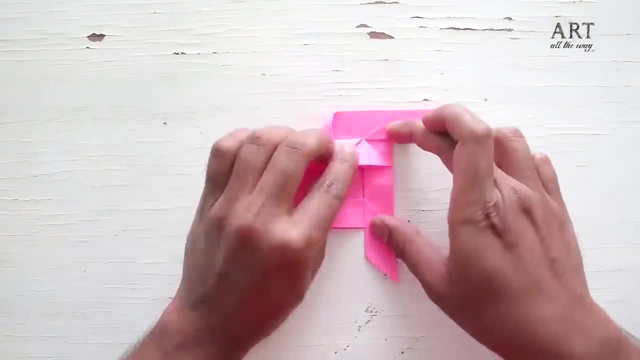 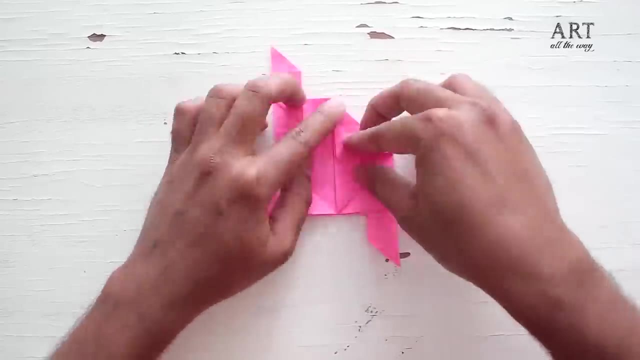 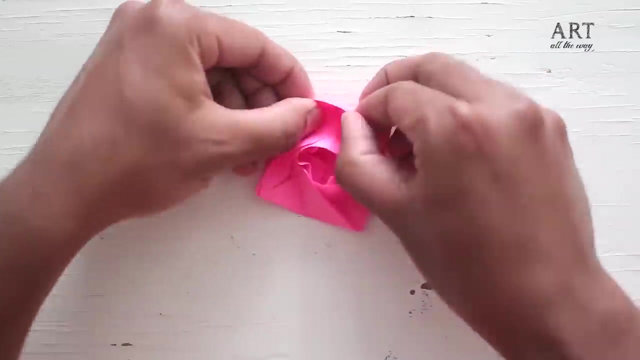 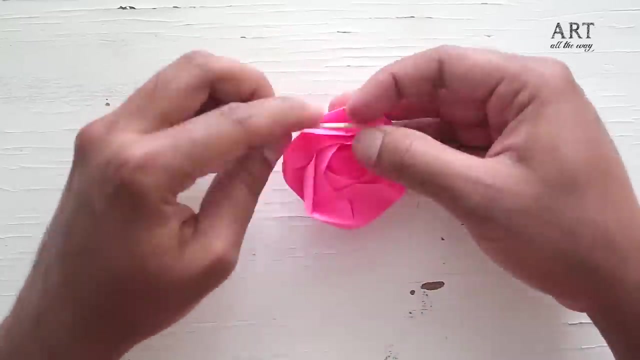 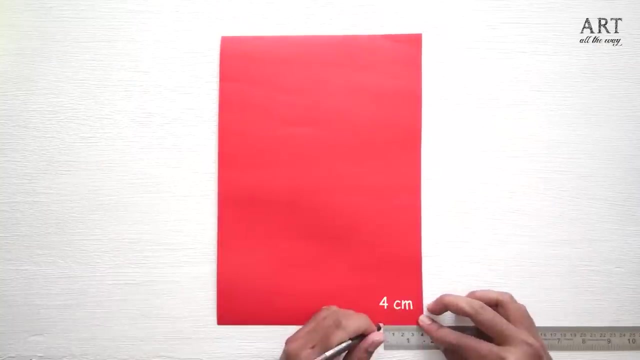 Oh, baby, as long as I got you. Oh, baby, baby, As long as you want me to, As long as I got you. You, you, you, you, As long as I got you. We faced the dark like if we weren't scared Close to each other's backs without no fear. 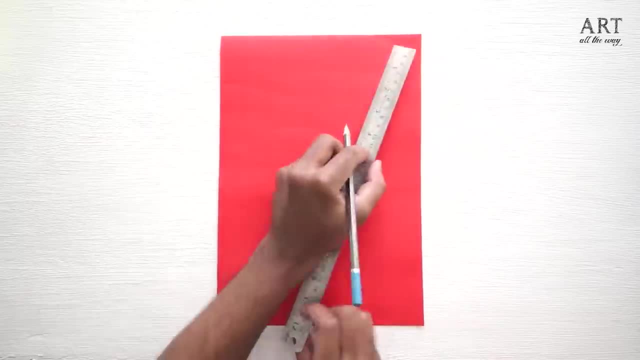 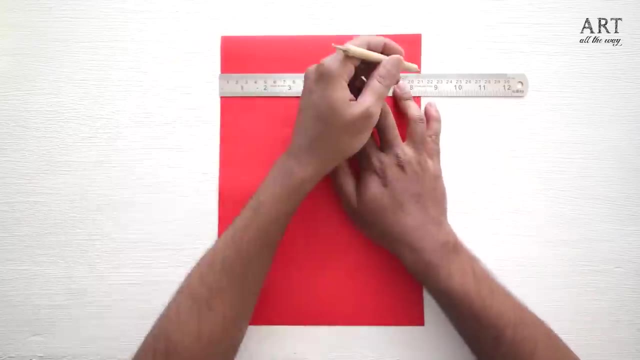 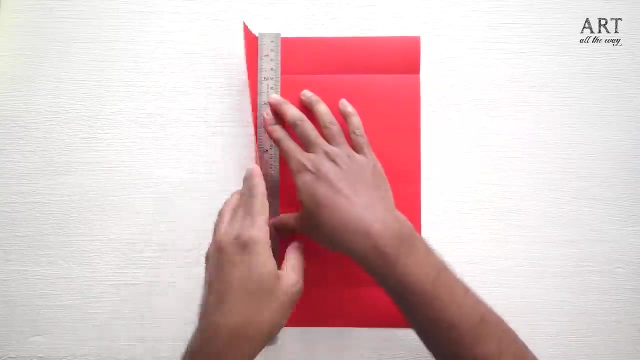 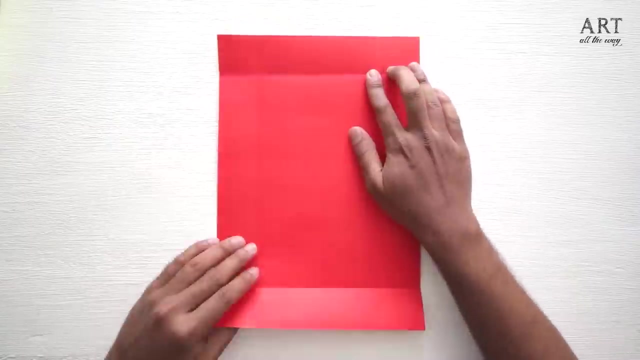 Hold on and waited for the sun to appear. Cause in the nighttime, I'm by your side. Oh, baby, when you hold me, I rather lost my senses Than be lonely. Cause, baby, when you touch me, I feel holy. Oh, nothing in the world would. 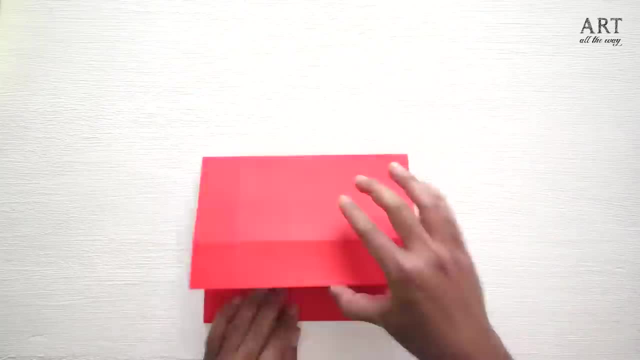 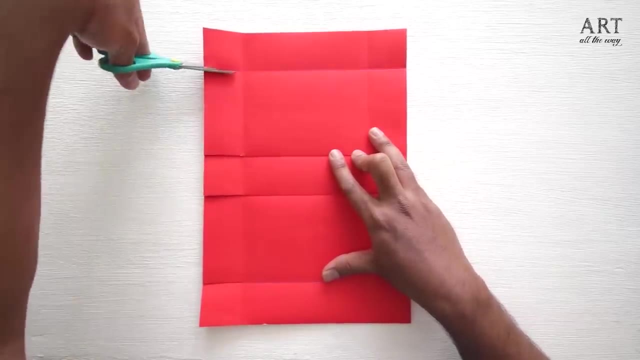 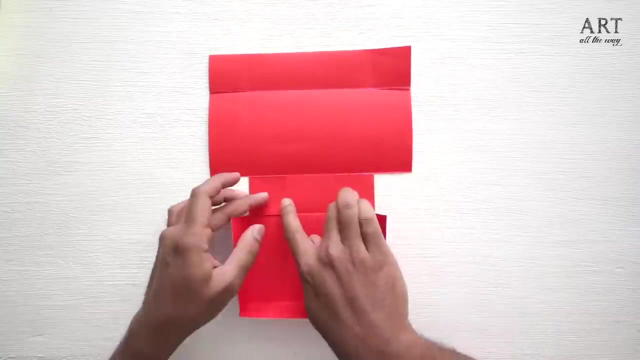 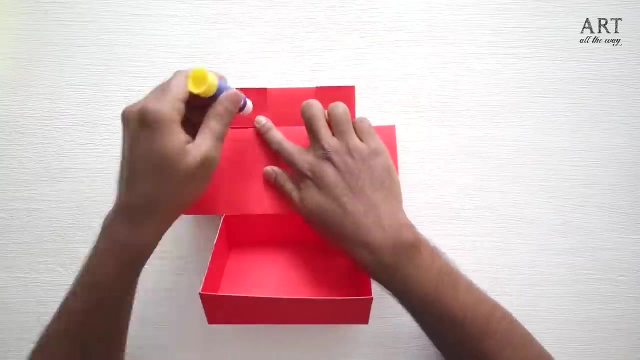 Oh, would kill me. As long as I got you. Oh, baby, as long as I got you. Oh, baby, baby. As long as you want me to, As long as I got you, You, you, you, you. As long as I got you, I'm done with the brain. 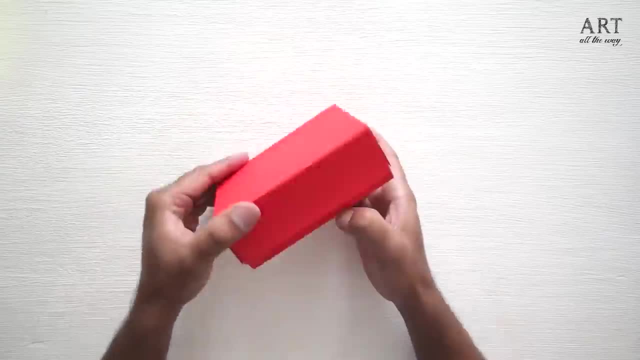 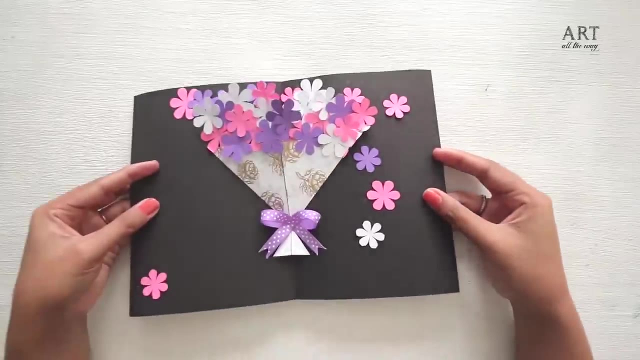 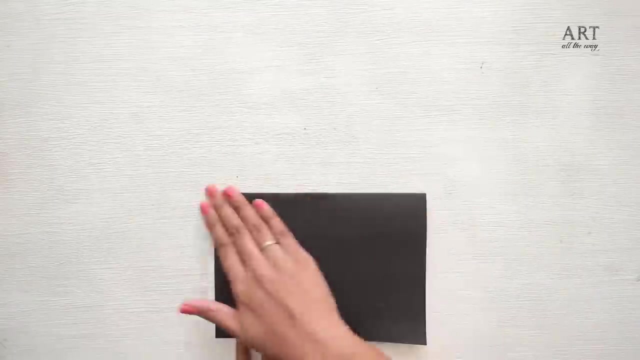 I'm done with the brain. I'm done with ache Cause. I'm done with fake As long as I got you. I'm done with embrace. I'm done with ache Cause. I'm done with fake. Oh baby, when you hold me, I rather lost my senses. Than be lonely. Cause, baby, when you touch me, I feel holy, I feel holy. Oh, nothing in the world will, Oh, will, kill me. As long as I got you, I'm done with embrace. Oh, baby, as long as I got you, Cause, I'm done with fake. 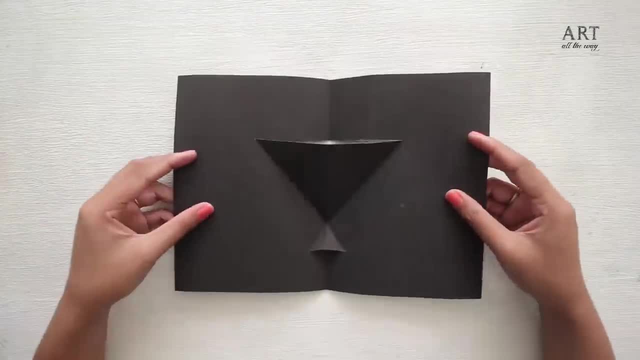 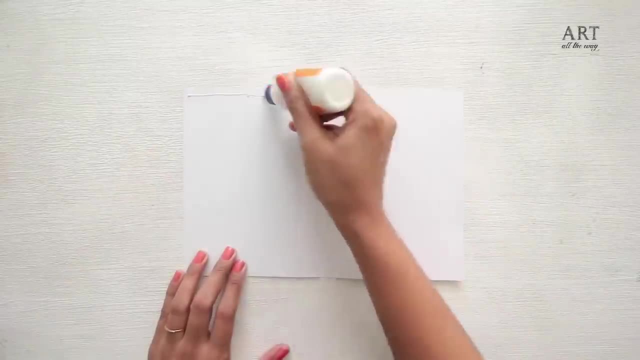 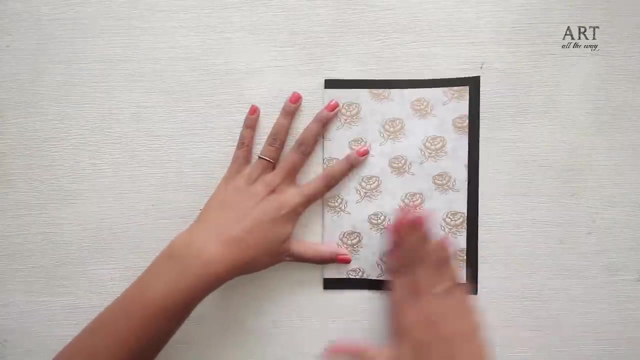 Oh, baby, as long as you want me to, I'm done with embrace. As long as I got you, You, you, you, you, As long as I got you, You, you, you, you, Baby. now, what can I do When the feeling's getting stronger? 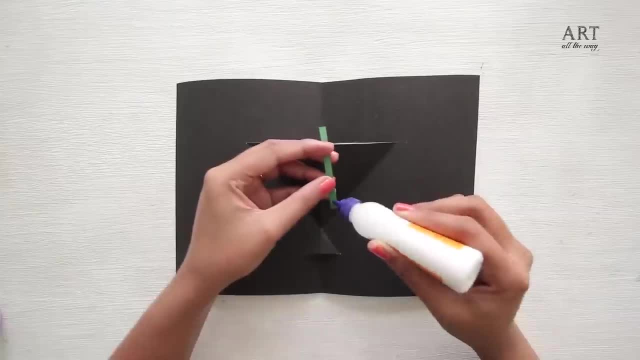 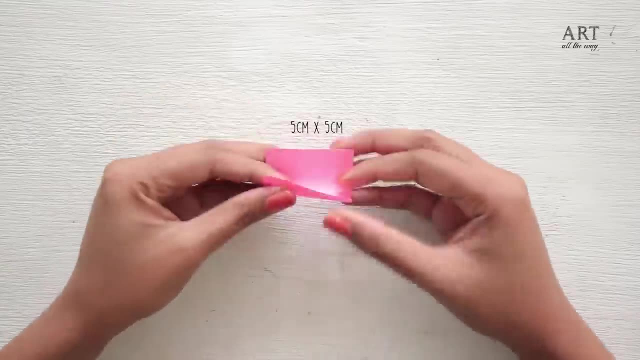 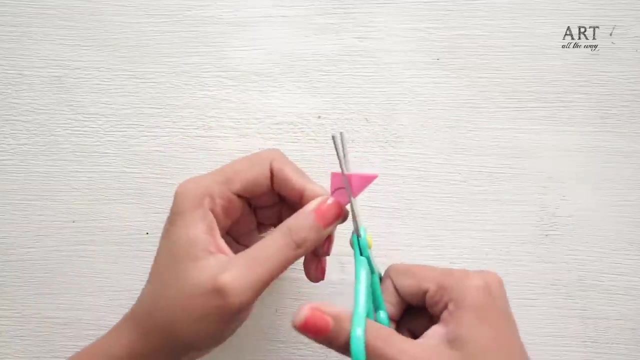 And the way that you move. I can't take it any longer. I'm addicted to you. Oh, I love it when you're looking at me. I'm addicted to you. Let me show what I got for you. Oh, I put this on you, Never mind the pueden. Never mind the disponibles. So won't you come along? together we're stronger. the night ain't really over. So, baby, come along, sit back, relax, turn off your phone and I will make you feel at home. So, baby, come along. why won't you come along? 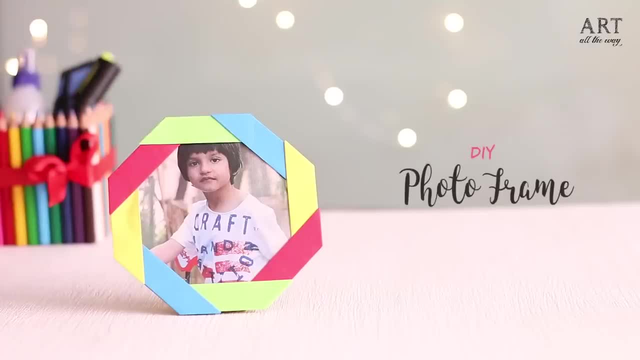 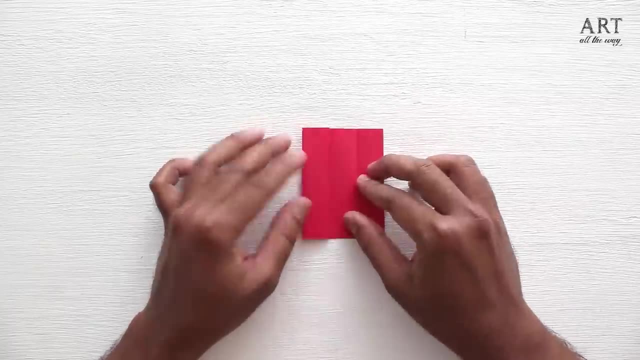 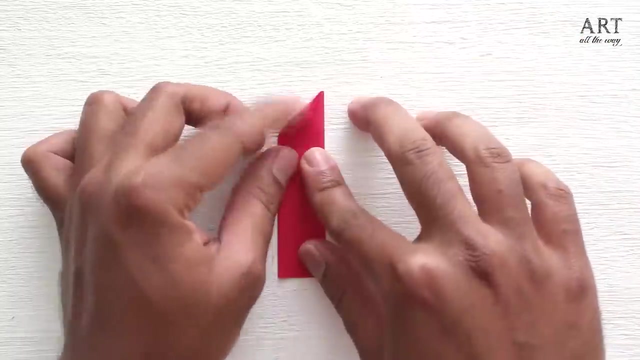 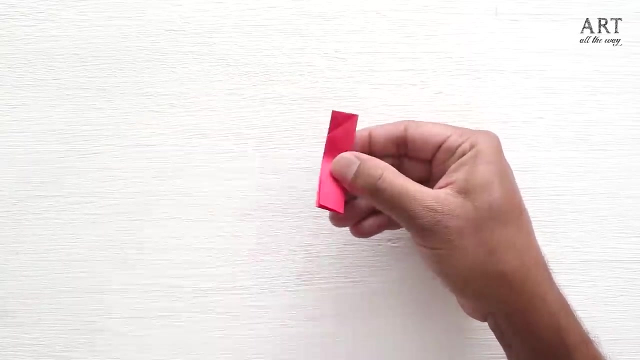 So what you say might seem a little crazy. Let's drive away. oh, you're looking so amazing, I'm addicted to you. oh, I love it when you're looking at me. I'm addicted to you. ha, let me show what I got for you, girl. 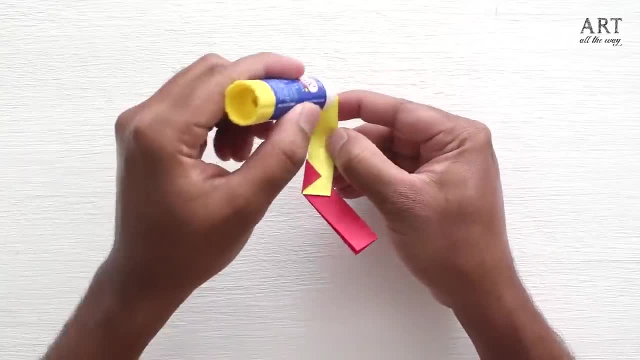 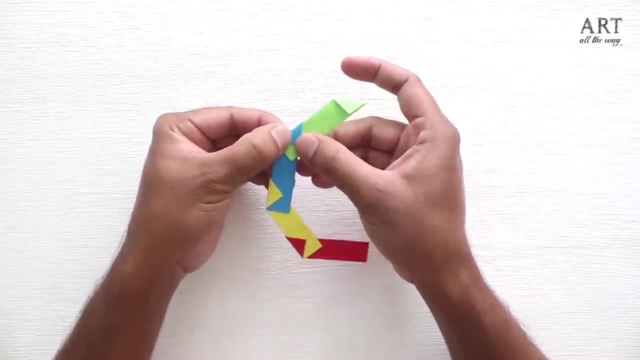 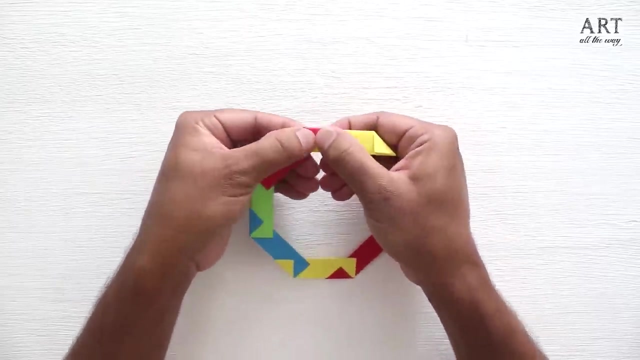 So won't you come along? together we're stronger. So, baby, come along, sit back, relax, turn off your phone and I will make you feel at home. So, baby, come along, sit back, relax, turn off your phone and I will make you feel at home. 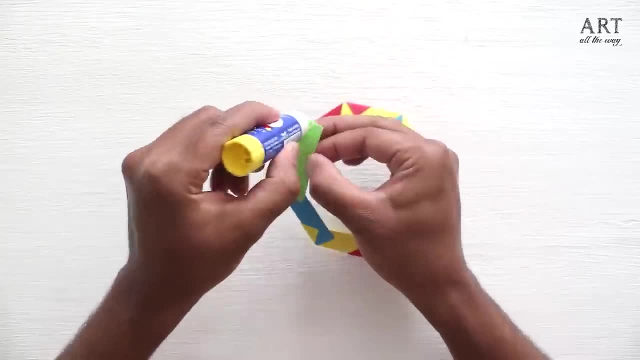 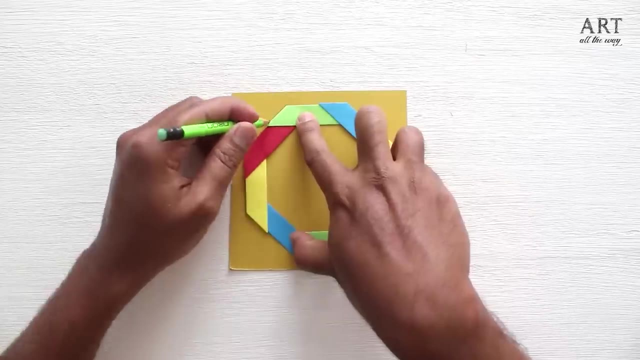 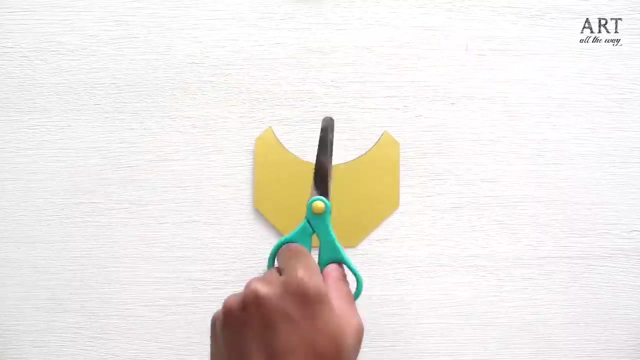 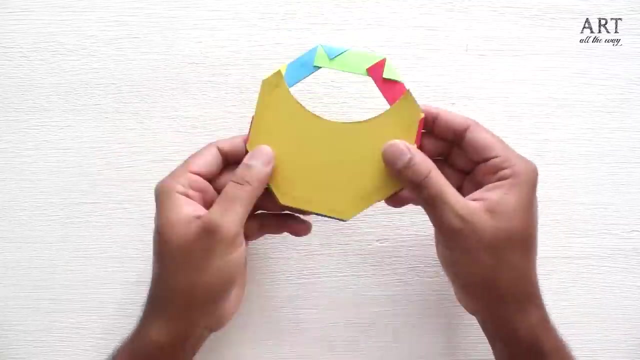 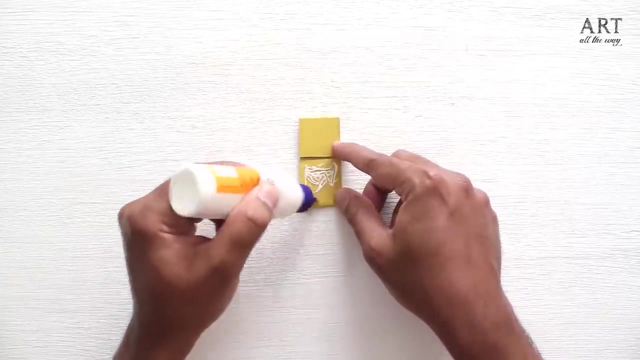 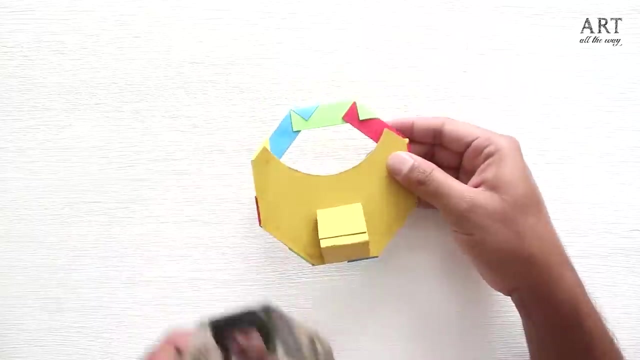 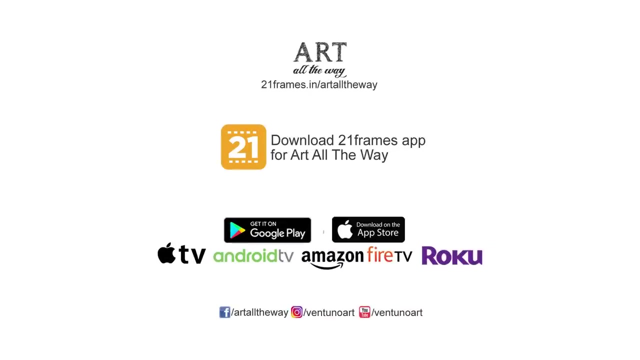